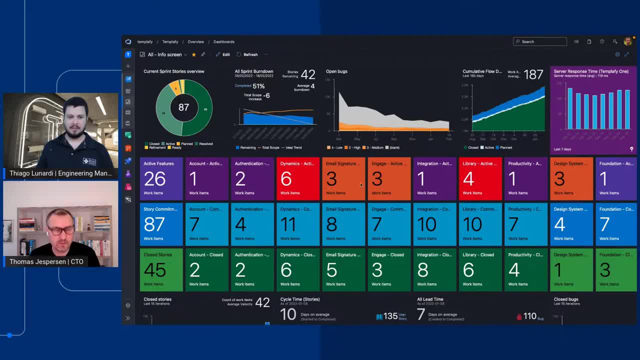 you can see is that every single team, every single product team, can see how many active features they have, how many stories they have in the current sprint and how many stories they closed. So these are our life right. It is a real deal. Yes, So this is, this is real time updated And 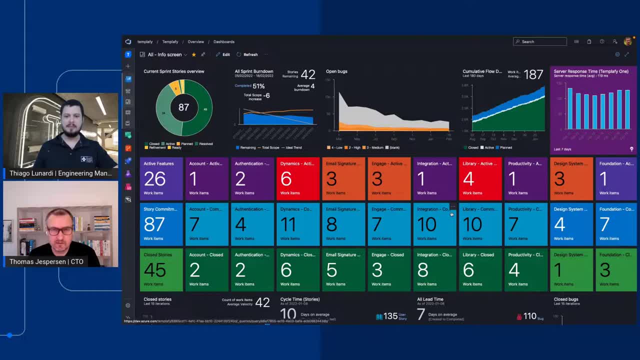 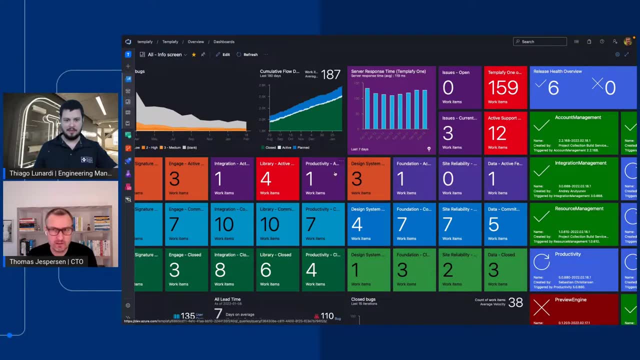 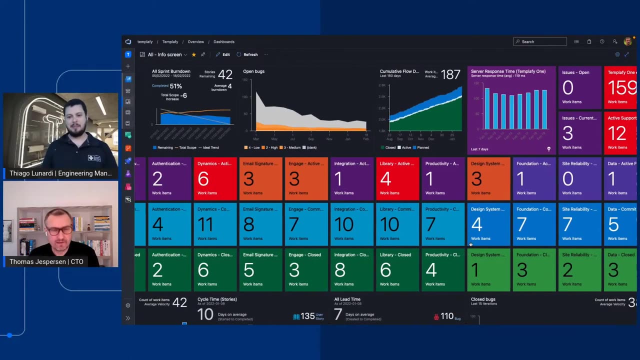 every single team has a column where they can see the status of their current sprint And if you scroll a bit to the left, you can see the platform teams which are serving the product teams And you can also see status of our bill And you can even see there's a failing bill down here. Yeah, happens. 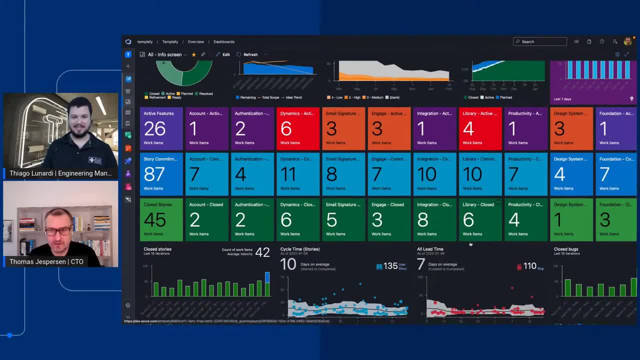 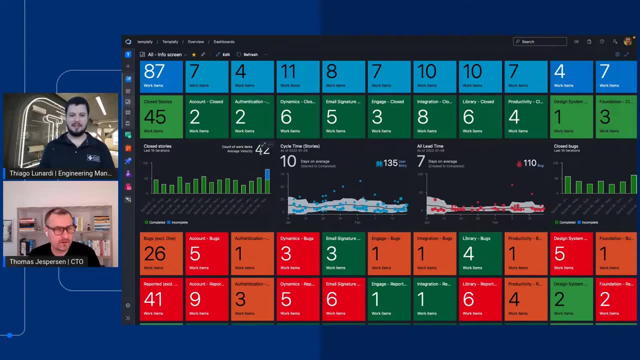 It happens. So you can see this is. this is not fake, This is real. If you scroll down a bit you can see a historical overview of the stories we close. we close 42 stories on average per sprint across all teams. average cycle like time is 10 days. you can see we fixed 110 bucks this. 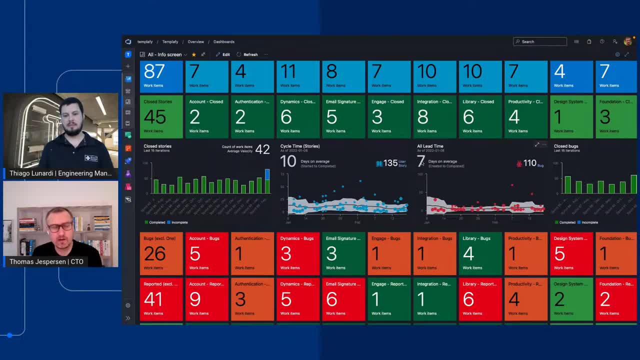 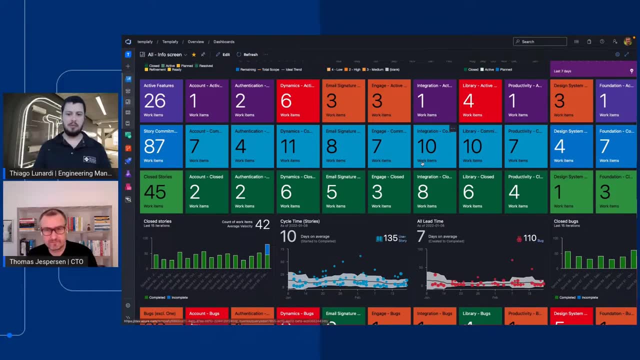 year And the lead time is seven days from a buck is reported until it's fixed and running on production. That's a good camera right. All the engineers are doing a really good job on that matter. We have been guessing a lot, We Yes, as you can see actually up here. 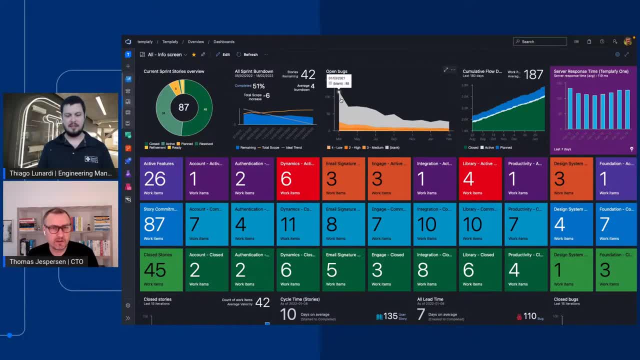 this is the how the buck has evolved over the last year. So I think a year ago we had 100 bucks And now we are down to 26 bucks in our system. So there's really a lot of focus on, on the, on the. 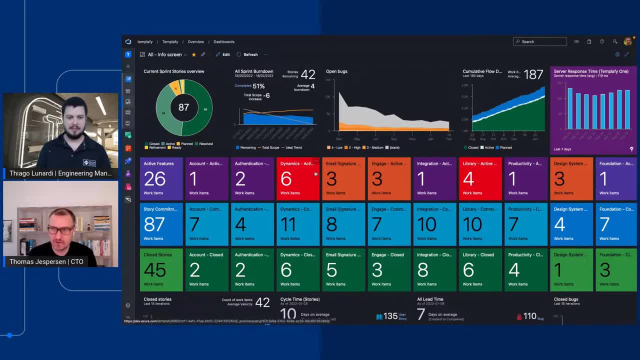 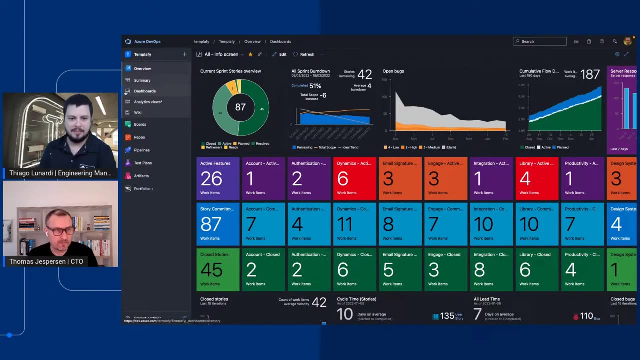 quality, And I will come back to why. because we do a lot of deployment, So we really need to focus on quality. Cool, So let's see in the team scope how it's working out. Yeah, so let's start by just having a quick overview of DevOps as a DevOps. So there's an overview. 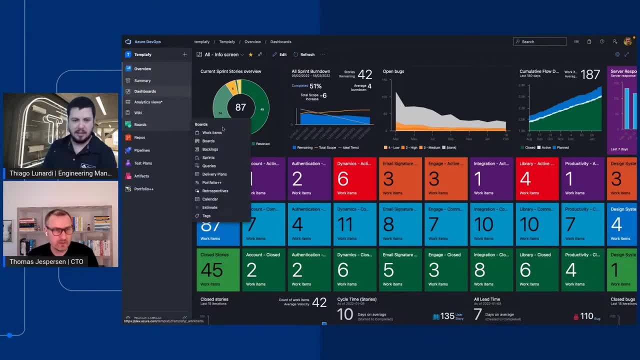 I just showed you the dashboard. then we have some boards where you can see work items and backlog and and sprint backlogs. We'll come back to these repository. This is our git repositories, like files, pull requests, branches and so on, And we will also show you our build pipelines. But 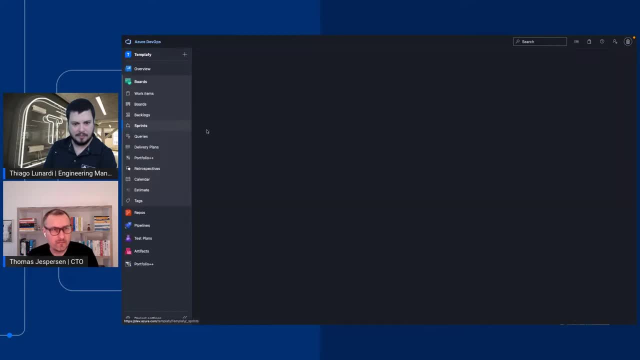 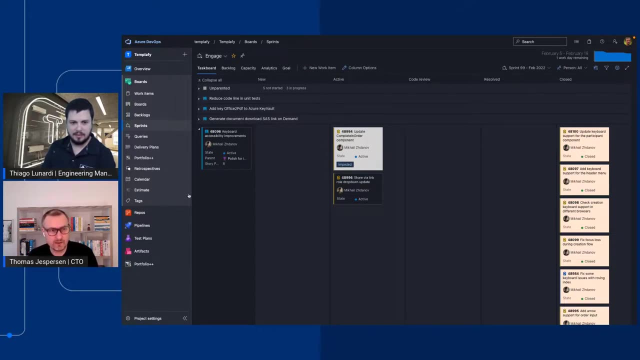 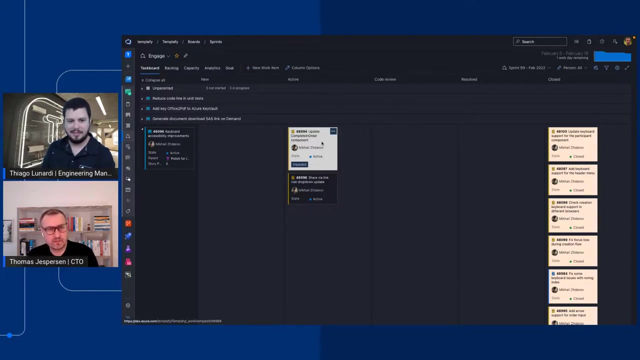 let's start by actually go into a backlog or a sprint board for one team. So I believe this is the engaged team that you are manager, And what we have here is a story, And a story is broken down to different tasks, And every single one of these tasks is actually a deployment to production. 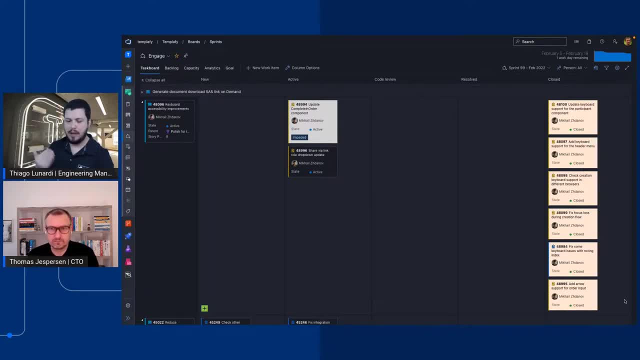 So every time that you make a change, should be ready to go to production, right? No, we follow the DevOps principles, So this and the lean principle about small batch sizes, So every single task is all the way to production. And let me show you how this happens in a safe way, where 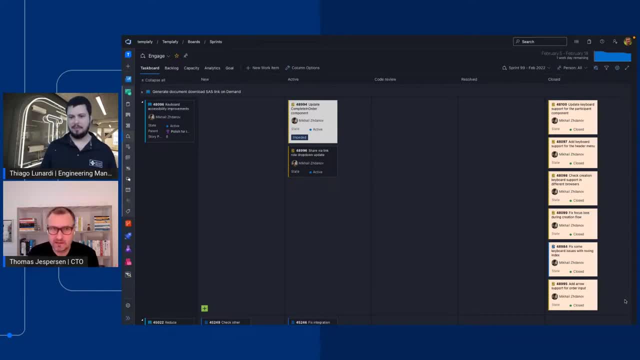 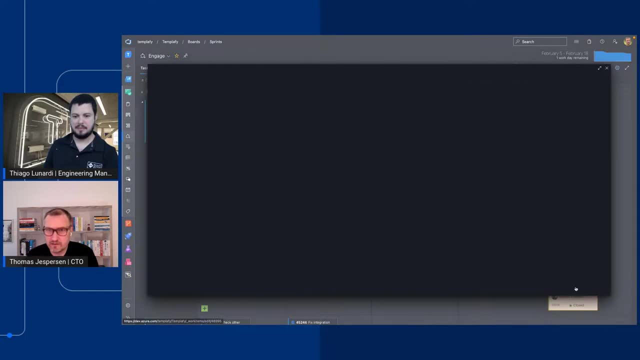 we can still make sure that we don't compromise on scalability, security and all those things. So if we take this task here, which you can see is deployed two hours ago, And what you can see here is that that there's some development artifacts, And if I click on this one, I will go to the pull- 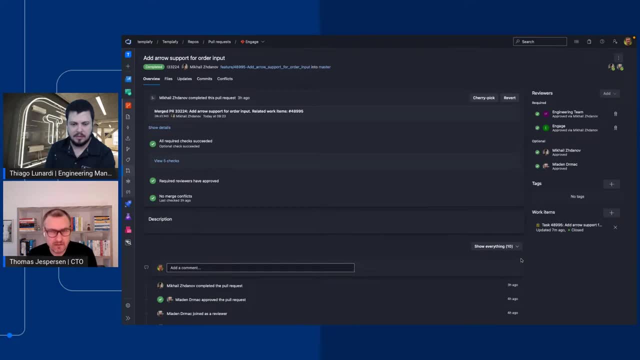 request that's behind this task. So this is the pull request And this is how it looks in DevOps. I can see that it has been approved by Michael and Im Mladen. There's some setup that says: because this is a change to the engaged system, it's a tool we have, The engaged team must approve. 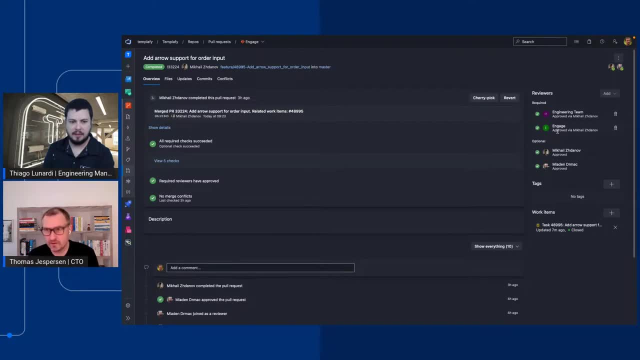 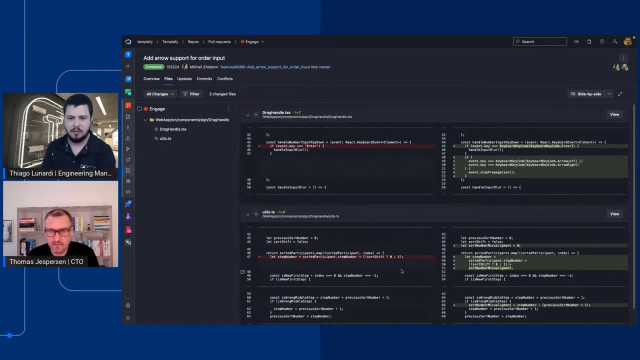 it, So no other teams can go and deploy your system. And if we just quickly look at what was in this pull request, you can see this is something about some keyboard shortcuts and it's not very big like two files changed and this is one deployment all the way to production, even though 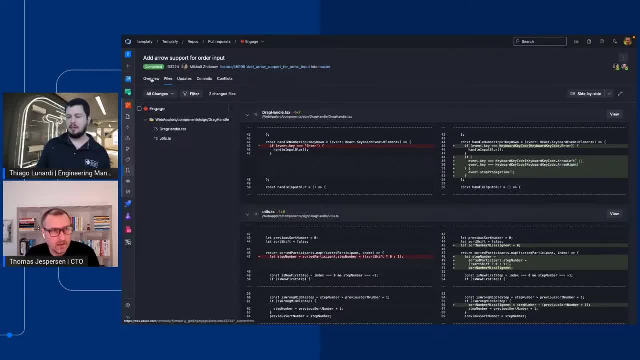 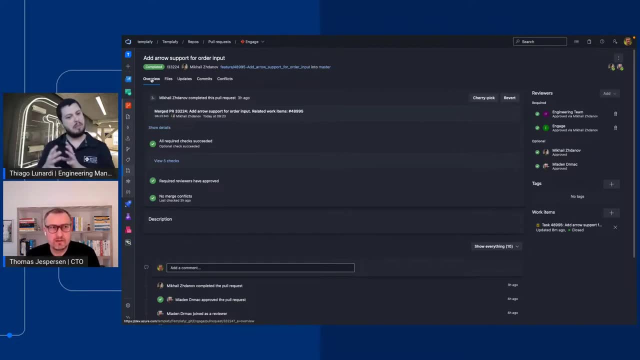 it's very small and what's the benefit that we are doing those tiny changes to production like so instead of piling up? so there's multiple benefits. it all ties back to some of the lean principles about small batch sizes and fast feedback, so you can imagine when we release. 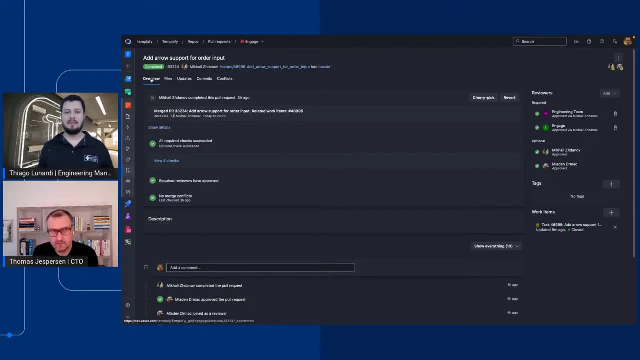 something like this: it goes to production. let's say that we introduce a bug or maybe even an incident. the great thing is that if we only released two small files now, we have an incident. how fast do you think we will discover it? rhetorical question: very fast if we batch it up in. 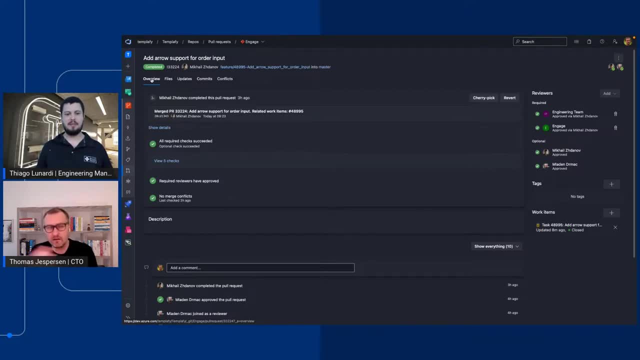 two weeks, there will be a lot of code changed all over the system and it will be much harder for us broke the system and hence also take much longer for us to fix it. so small batch sizes: even though it's, it's well, i don't know if it makes sense. it's quite in not intuitive for most, but it actually is. 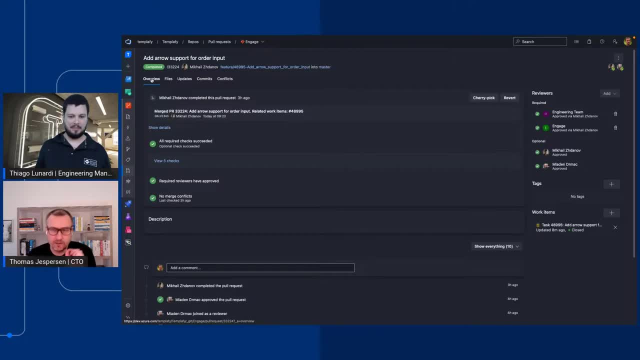 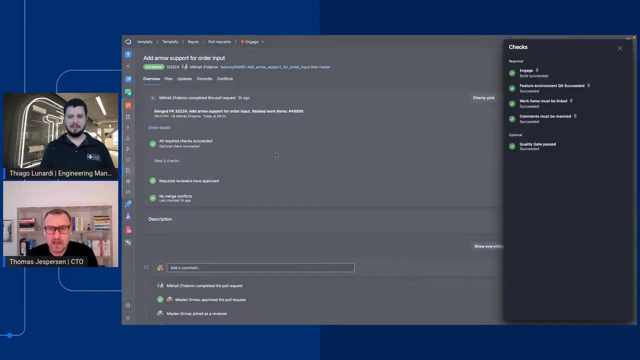 a more safe way to release software. so but to make sure we are not too, you know, over, over ambitious, we have a lot of checks for every single deployment. so first of all, of course, the build must run and the unit test must, must, pass. but we also, before we merge it down, we deploy it to a 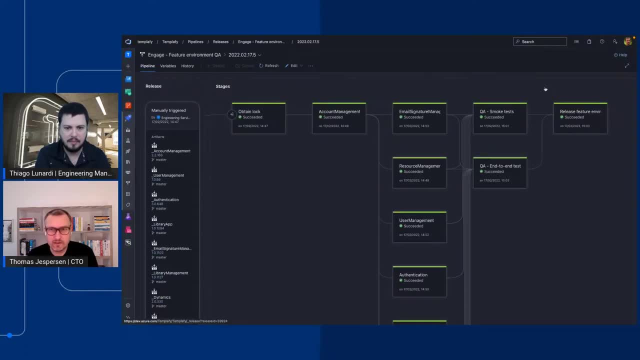 feature environment. so i will click in here and what you can see is that here we are running some end-to-end smoke test on a feature environment. so we take all the different systems in templify microservice, if you will. we call them self-contained systems because they're slightly 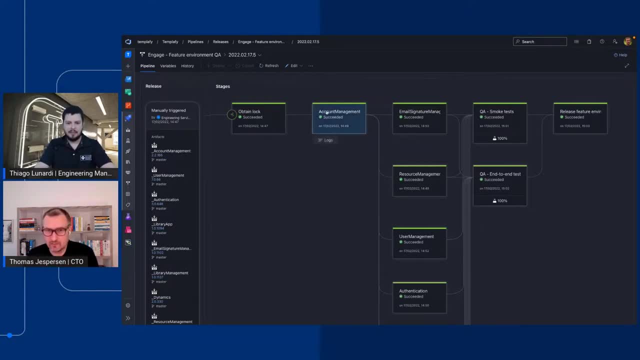 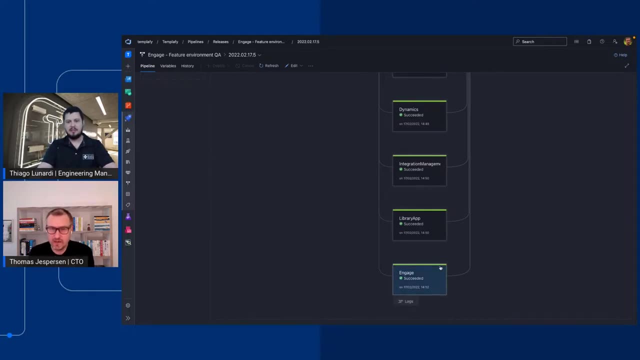 bigger. we have 14, and this is something like account management, user management, authentication, and then, of course, scroll down to the bottom. you will see you have engaged. this is your system, so we take the latest build from that is running on production of all the other systems. then we take a version of of of. 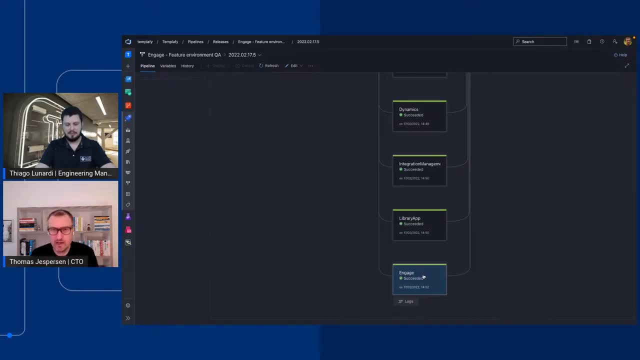 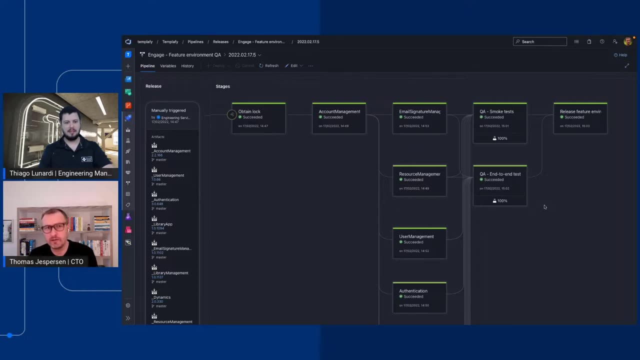 your system with the small little change with it, and we deploy it to a feature environment running in kubernetes, exactly the same as our production environment. it's all handled with terraform, so we know it's exactly the same types of services. it's the same type of message spots. everything is exactly the same. then we run some smoke test. 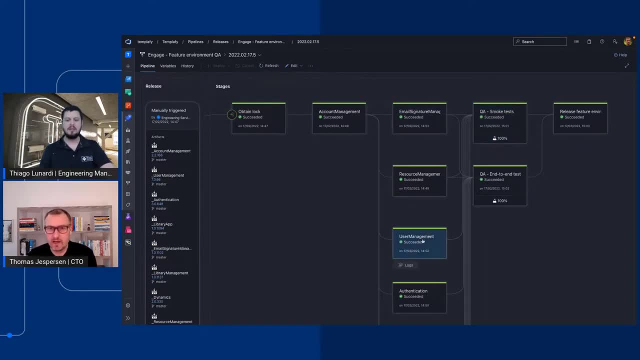 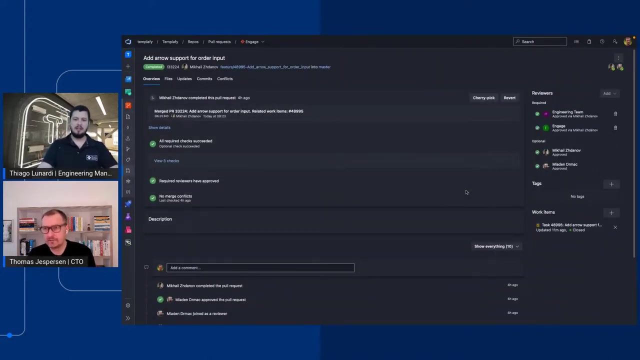 which makes sure that we didn't break any of the other systems, and we run some other end-to-end tests, which is specific for the engage team, where we go into new degree details and make sure we didn't do any regression test in your system. so that way we now have a really good feeling that. 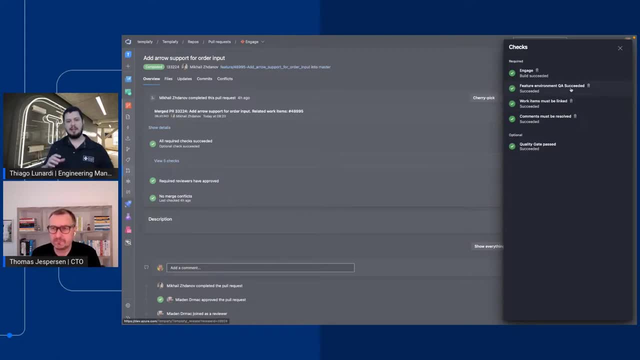 this is probably not going to fail on production, and exactly that, what bring us the maturity and also the bulletproof safety that we have to deploy to production every change, because we are covered with all this infrastructure and tests and all the way right. exactly, and, as you can see, these are required steps, so there's literally 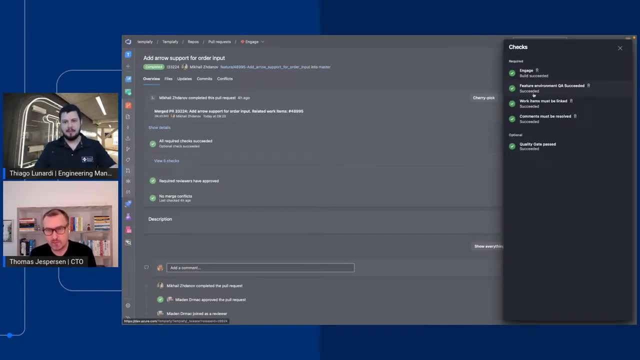 no way we can skip these. so even if we have a production incident, we don't skip the test. we still go through all these. so let's continue on seeing some of the other things we have here. first of all, there must be a work item link. i showed you the the work we actually started from. 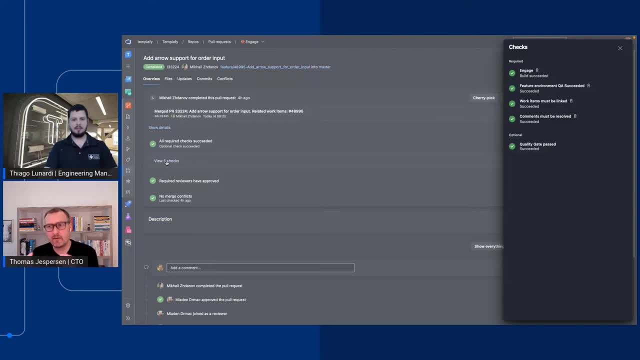 the work item. so so you cannot deploy without having a work item, which means, in turn, that we have full change management on who did the change and who created the, the change request, when was it merged, and so on. we'll come back to that. obviously, if there's any comments on the pool request, they 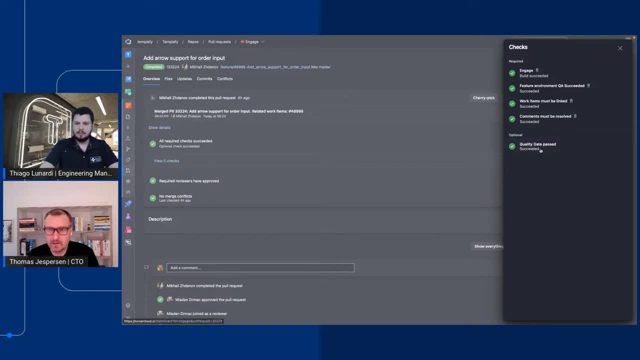 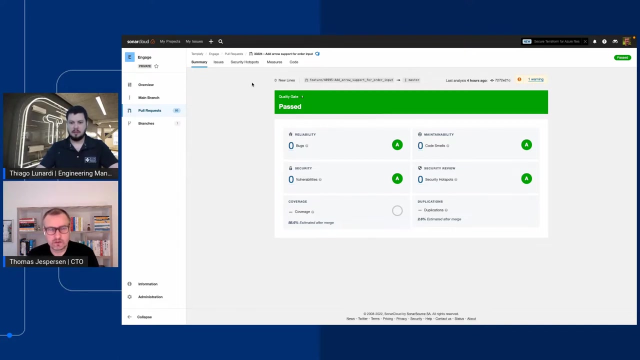 must be fixed. and then, finally, we have a very interesting thing here with with a quality gate. you can see it's optional. most the other teams have it required, but in your team it's optional. and if i open this quality gate i go to a tool called solar cloud. it's a software as a service- club service, where we run a lot of static. 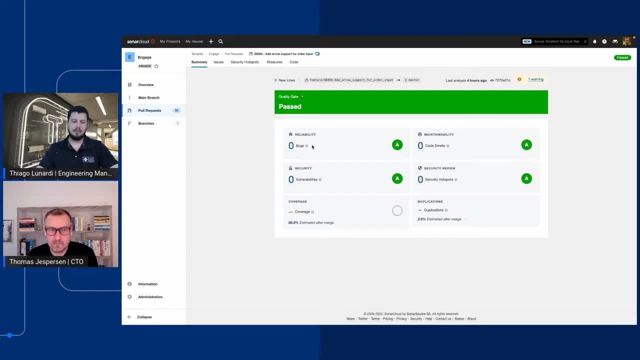 code analysis tests. so we test for bugs. it could be a division by zero. it will not make the code not compile, but it will be a runtime bug. it can also be more complex than that. it could be code smells. if you have too much, what cycle? magic complexity or tomorrow, or parameters, right, well, actually there's this. 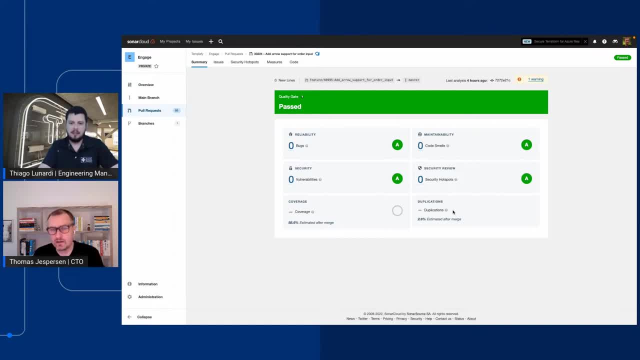 thing down here about duplicated codes, which is tracked is separately, because sometimes it's okay and, as you can see, there's some security checks. it could be something like a us using an md5 has and that's not really secure, or some security hotspots just okay. here we are actually using 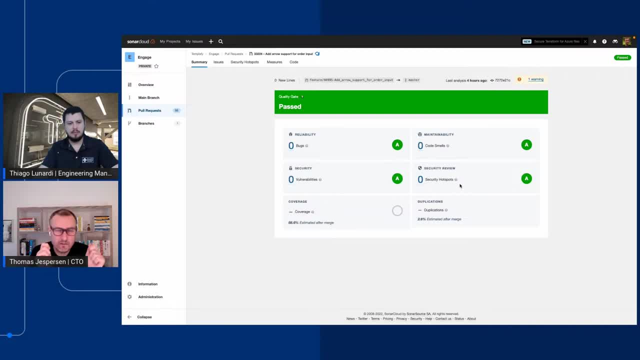 encryption and and and just make sure that all page page special attention. and the really cool thing is if, if sonar cloud finds any uh code smalls or any of these, it's actually going to annotate it back to the pull request in azure devops. so you as an engineer. 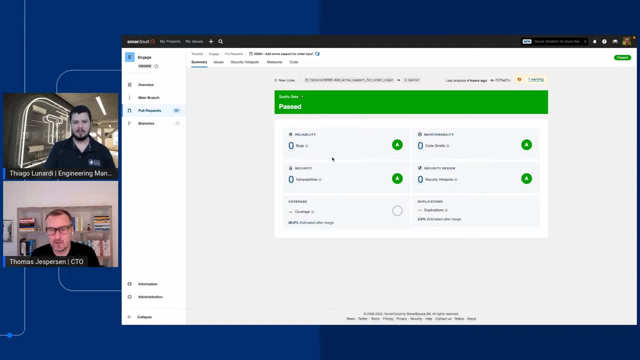 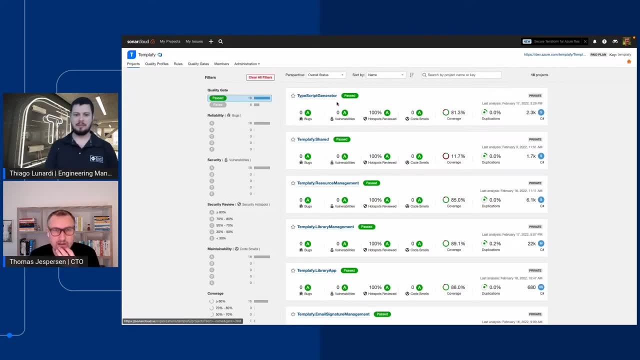 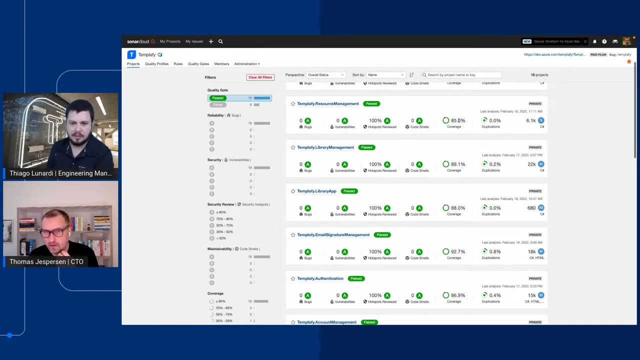 cannot merge. if there's any findings, well, you can ignore them, but we don't. we fix them and just to. if i go and look at all the different systems we have, you can see that These are all the different systems we have and there's pretty high code coverage on all. 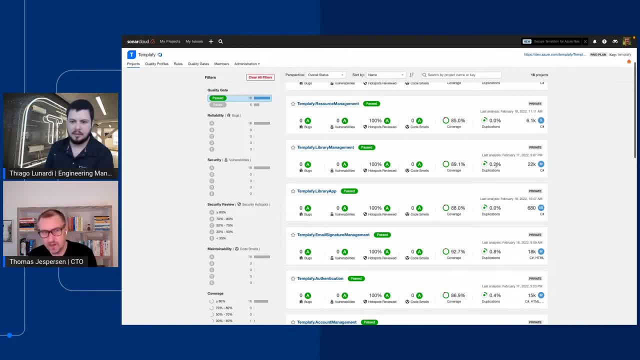 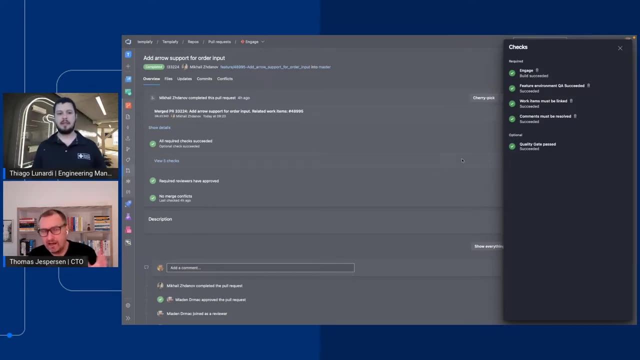 of them. You can see here the duplication. there's some, but there's no box vulnerability or code smelts in any systems. So pretty cool, And this is running every time we do a release And that's helped us to always deliver a really high quality product right. 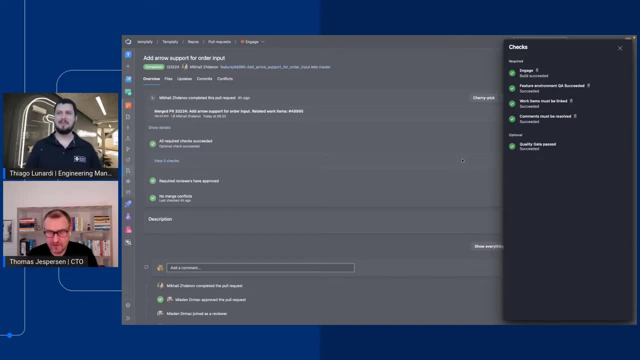 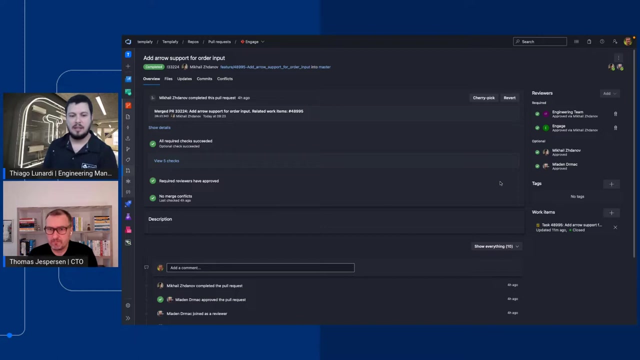 It helps. It helps. So it's not a guard against common sense and pair programming and all that, but it definitely makes sure that you don't do these stupid mistakes that a computer can detect. Yeah, definitely So. all this happens every time we have a pull request. 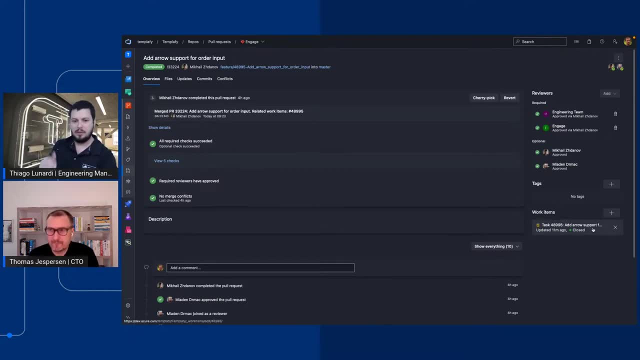 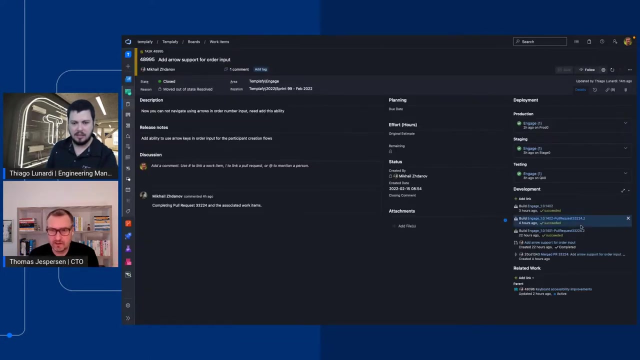 But let me get back And inside the build pipeline. I think we passed through it. Can we take a peek inside the build pipeline? that was a pull request. Let me look. It runs on the pull request. Let me actually go back to the work item here. that is, whatever it smelts down to main. 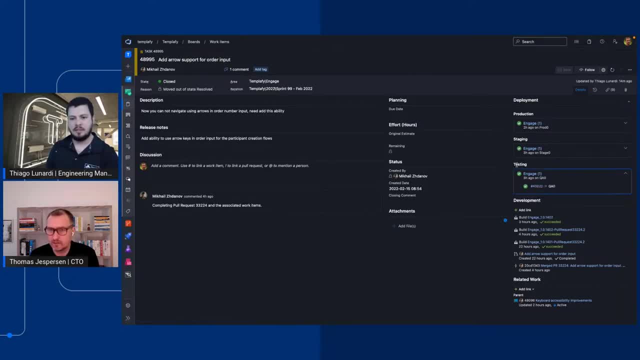 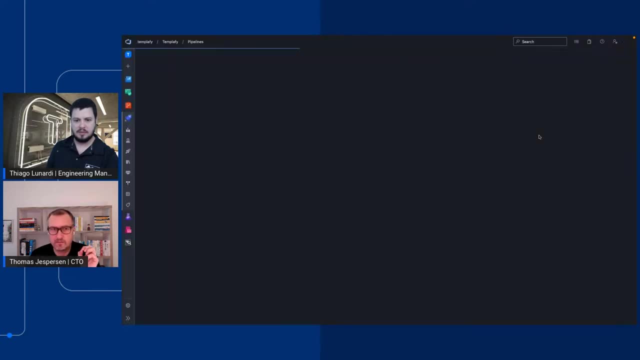 or master. it actually kicks off a deployment, first to our testing or QA environment, then to our staging environment and then to our production environment. And if I go in here to the production environment, you can see the first things that happens is that it kicks off a full build. 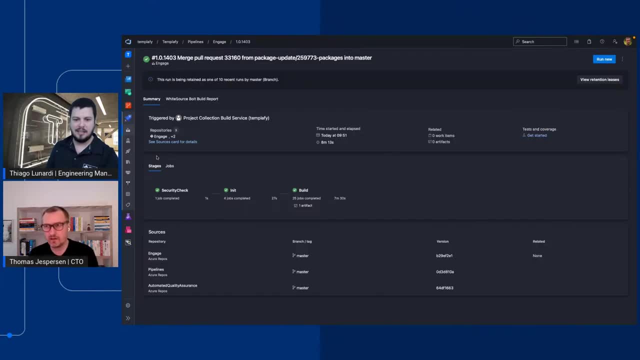 So I think what you are asking, too, is if I go into this field. Yes, exactly that. Here I can see all the different things that happens. So first there's some security checks, there's some versioning to make sure that every single 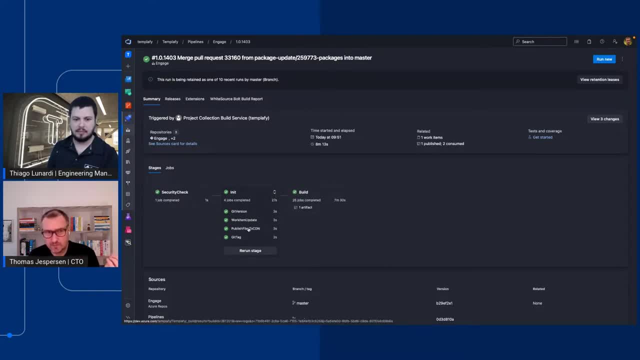 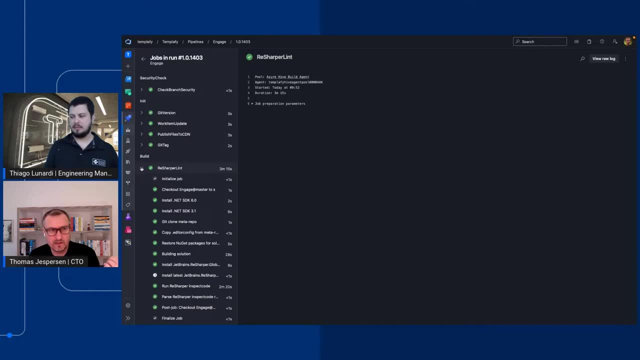 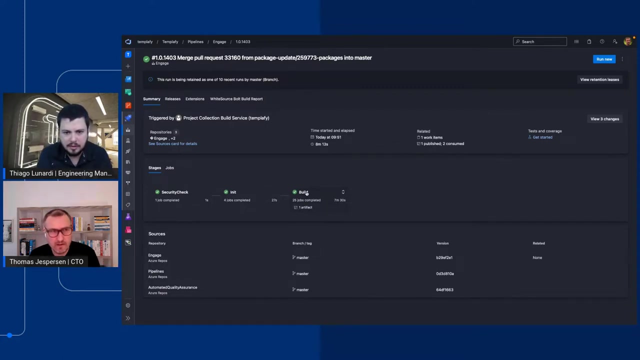 build has a unique version which is tagged in Git, and we publish files to CDN And I can deep dive into the build itself. So, as you can see, the build took- I think it was here. it took eight minutes in this case, or seven minutes here. 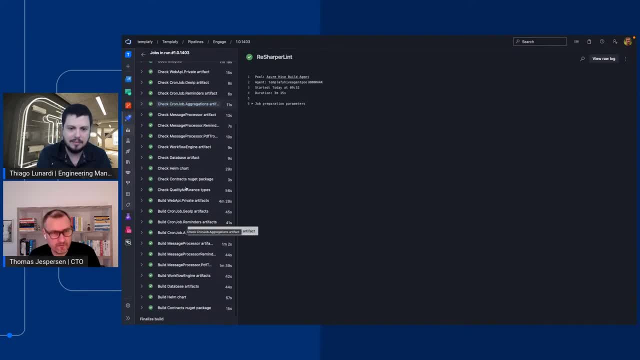 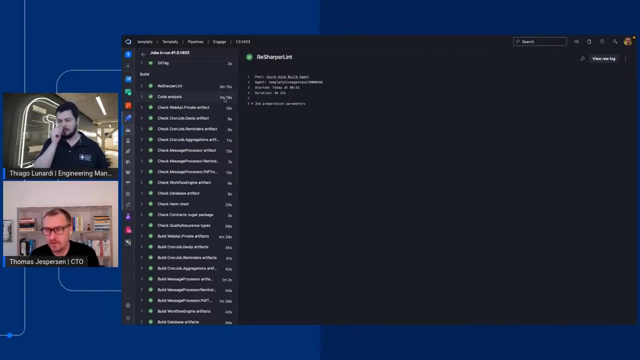 And if I look in, you can see there's a lot of different things happening. There's some code analysis, the static code analysis that we just showed you. it's fairly slow, It actually takes all the time, almost all the time, but still in parallel we have different 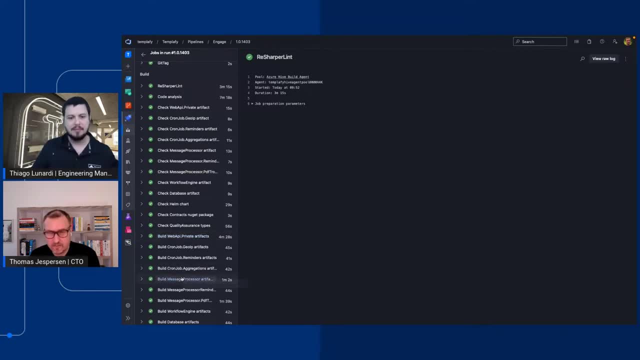 things that's running like build artifacts and different components in our system, And we also have this very interesting things here called ReSharpa lending. You may know ReSharpa, which is JetBrains developer tools. We use that to develop And there's a lot of code conventions that 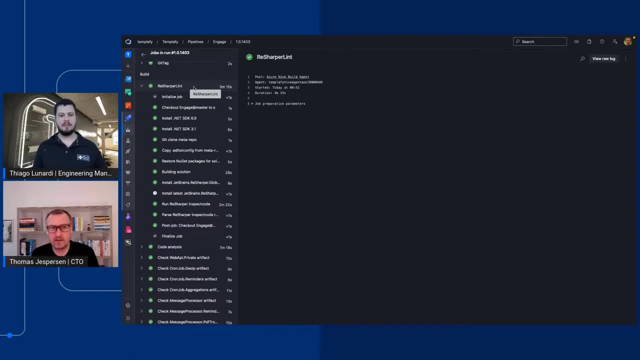 There's a lot of code conventions that we have enforced, like spacing and using VAR over the types. it can be how we name our parameters and variables and so on, And this is running every single time we make a deployment. So you cannot even make a deployment if you are not following our code conventions. 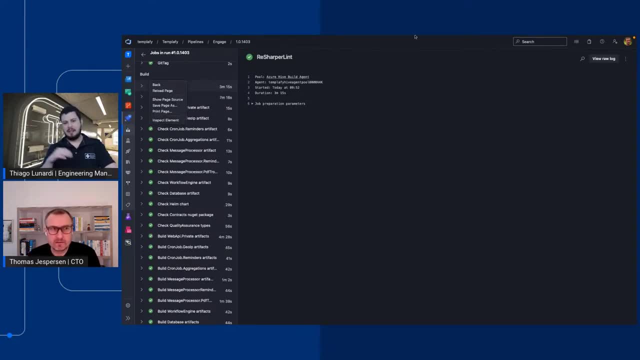 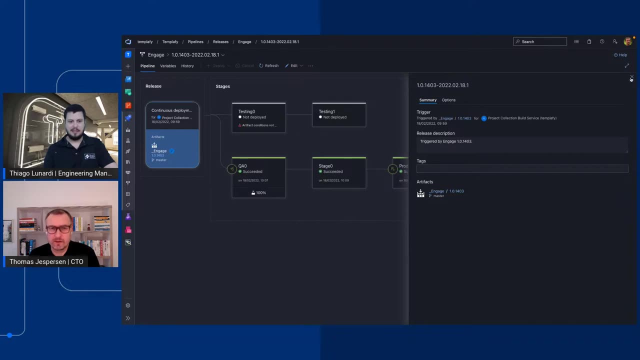 Awesome, Yeah, And that should run forever. It should run forever, right, Because one is running for six minutes, seven minutes, four minutes, So I'm not sure what you mean. Yeah, As each task inside the build they run for over five minutes. 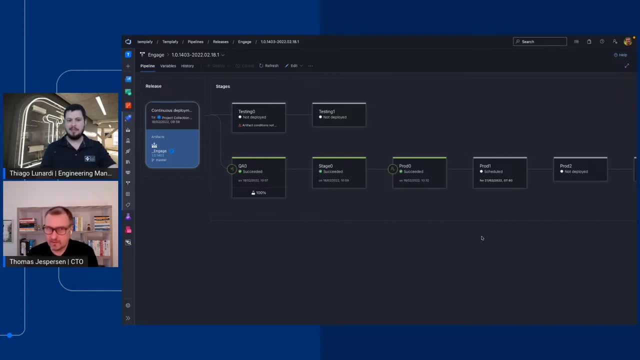 So all those collections should run for what in a half an hour? Well, yeah, because, as I showed you the final, the entire build took like seven or eight minutes. So they run in parallel to make sure that we speed it up. 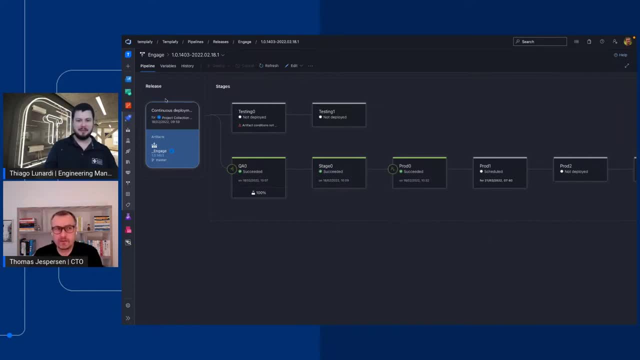 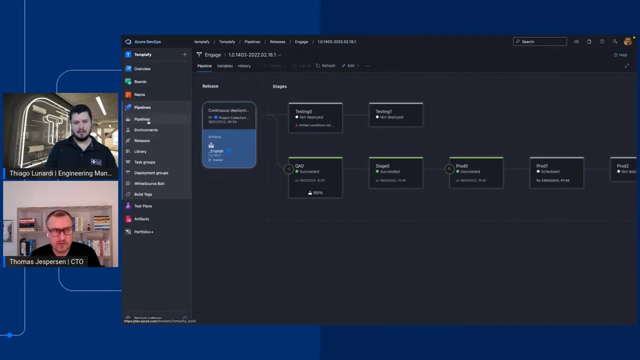 All those workload, Yeah, Yeah. And then, once the build is run, we kick off a release. And some of you who are DevOps fans might say: why are we using the release pipelines to doing a release? Because if we use these Azure pipelines, you have the YAML files and version controls. 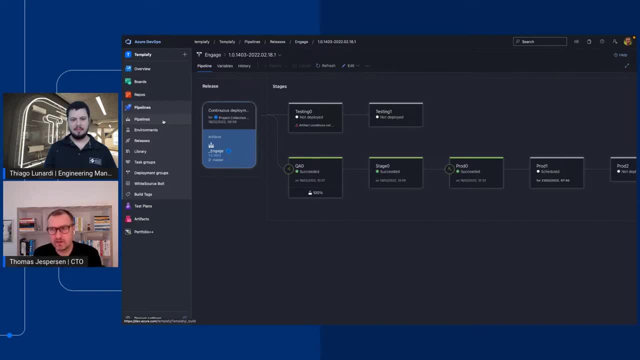 And you would be right. That is the direction Microsoft is, or was going, at least. But one thing we get by using the release pipeline is this very nice integration that I showed you, Where I can click. I can go back to the instance here on the QA and I can see what work items are deployed. 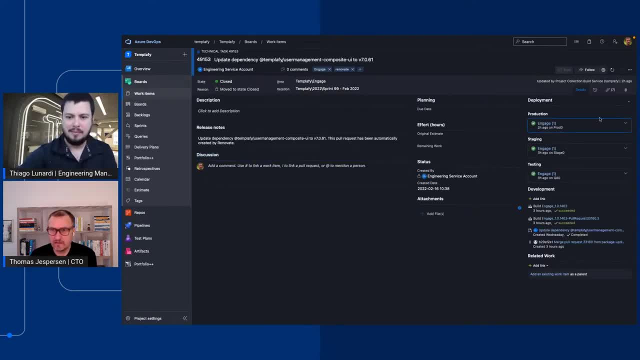 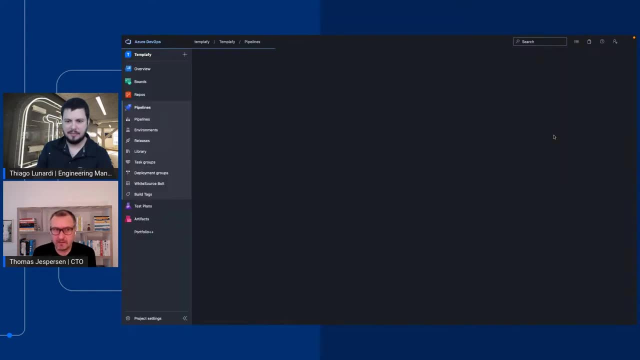 So I can go in here and go back to the work item, And it's kind of like I'm going in circles right now, So I'm back to the work item and from the work item I can go back to release on you. 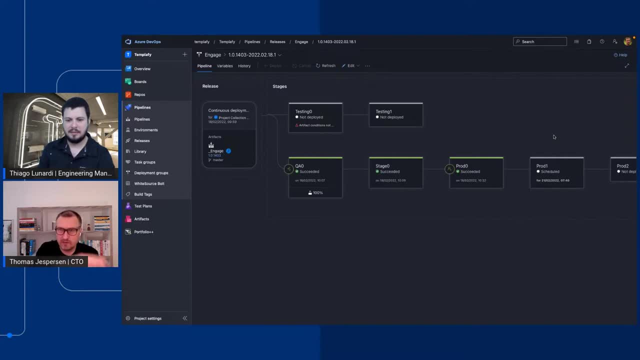 know I can navigate both from the pull request to the work item to the release or from the release to the work item to the pull request. So it's all kind of tied up And that's what you get when you use these release pipelines. 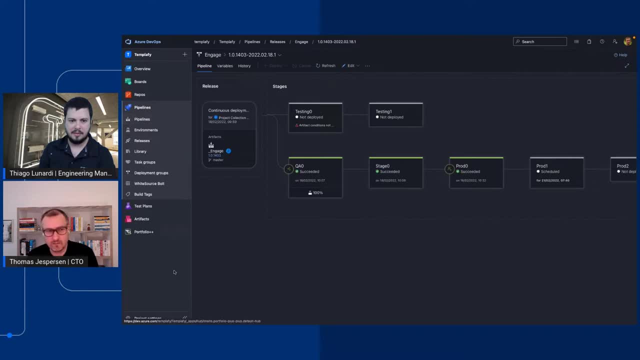 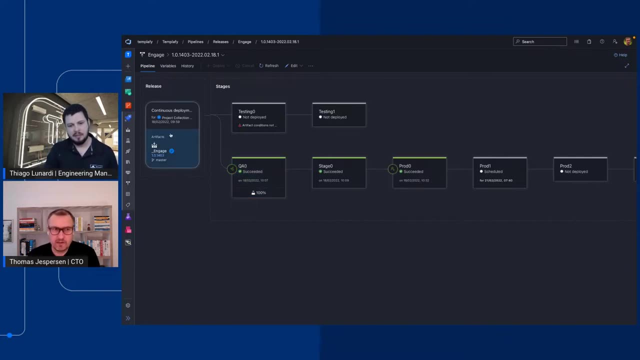 Which you Cannot currently get with the Azure pipelines. Then we have the deployment to QA. So after the build succeed, we deploy to QA And you can see there's a small pre-deployment check here Which means that we cannot deploy to QA unless the work item state is in the salt. 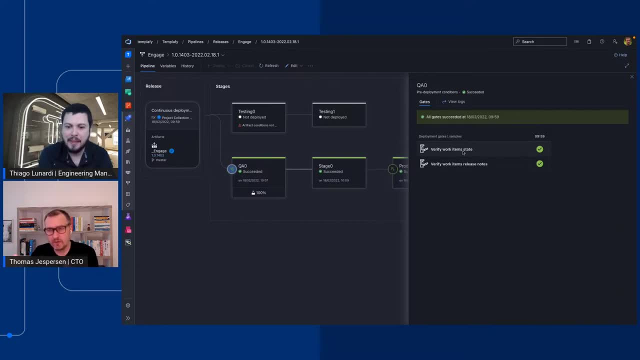 So this happens semi-automatically when you complete the pull request. When you create the pull request, the work item goes to code review. When you complete the pull request, it goes to result, But if someone tampered with it, it will not deploy to QA. 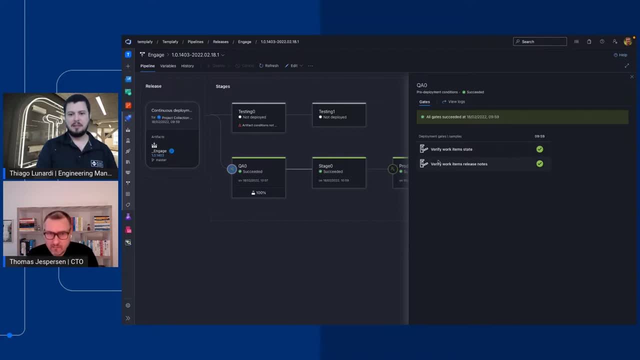 So it must be in the salt. Then we can also see there's a requirement. sorry, no, it's fine, Like it's really exciting to see a lot of that. I just don't want it to interrupt. So yeah, let's just continue. 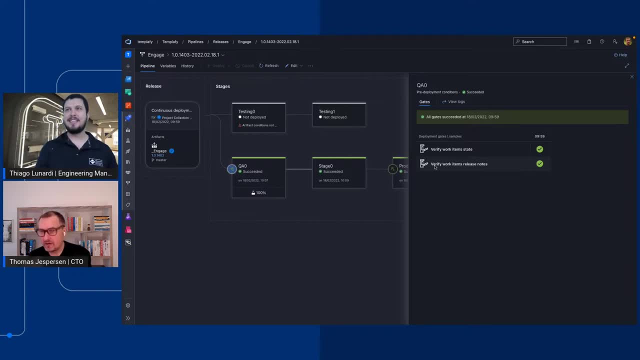 So here you can see there's some work items or some work And another check that says there must be release notes. So if I go back to the work item that is behind this deployment, you can see there's some release notes here And I'm actually not sure. 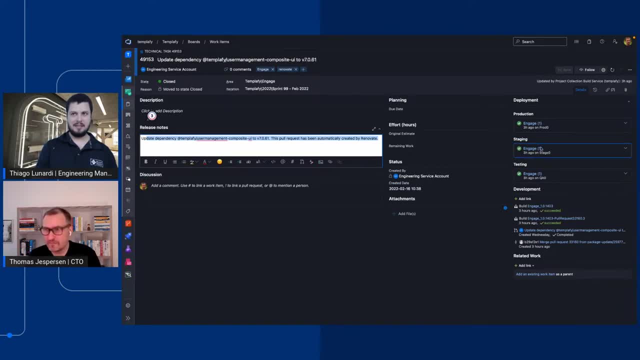 I think I ended up on a different one than I started out with after all, But never mind. Here's some release notes And I can take this number here and I can go into our Wiki And all these. every time we do a deployment, we publish the release notes. 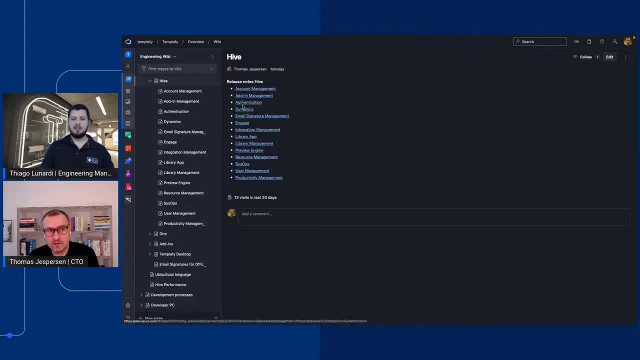 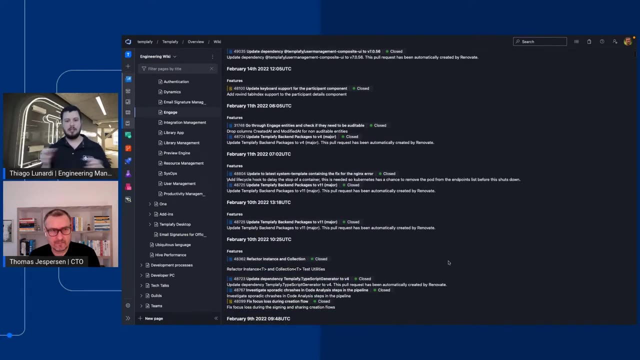 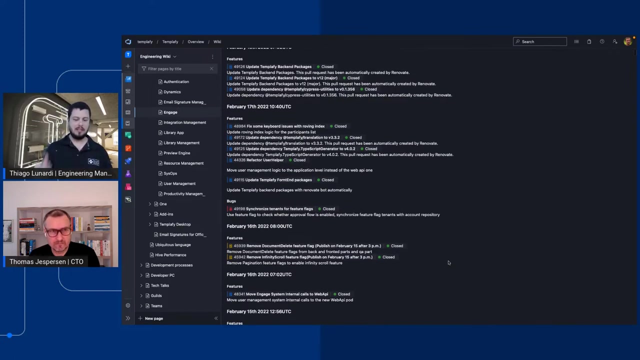 The release notes to our Wiki And we also publish them to a Slack channel, So the release notes that all engineers needs to add for each change. it's not there just for silly documentations actually being piled up in a common area inside this product, inside. 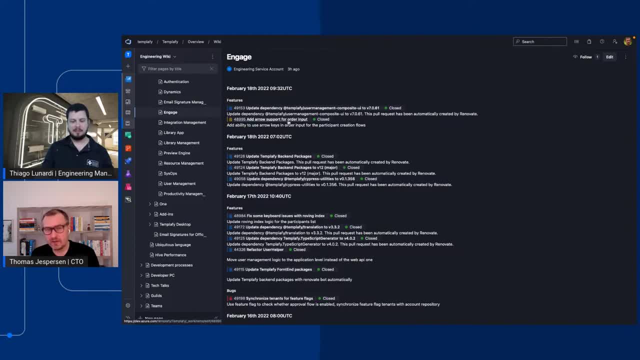 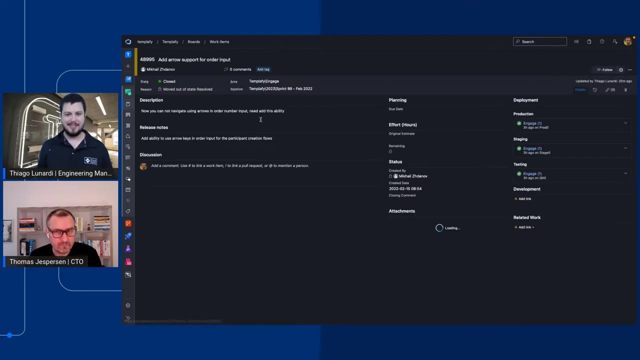 this week page right? Yeah, exactly, So you can go in here and then you can have a full list of all the changes we have. So, actually, going back to the original Yeah Task that we started out with- I'm not sure how I ended up on a different one- 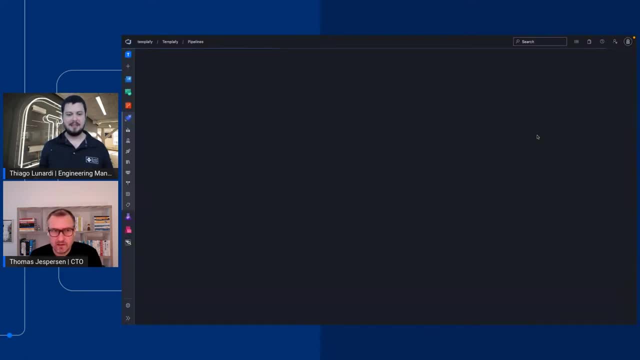 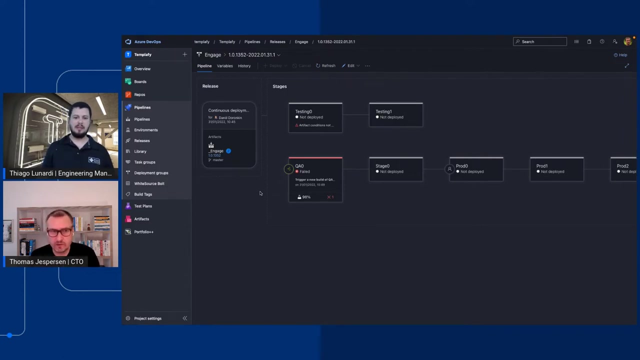 I'll just go back to the release here. So now it's running on QA and you can see that here we are also running the end to end test. But in the case that is actually failing, we have a video recorded. So I'll just go to a failed build, because only if it fails we'll do this. 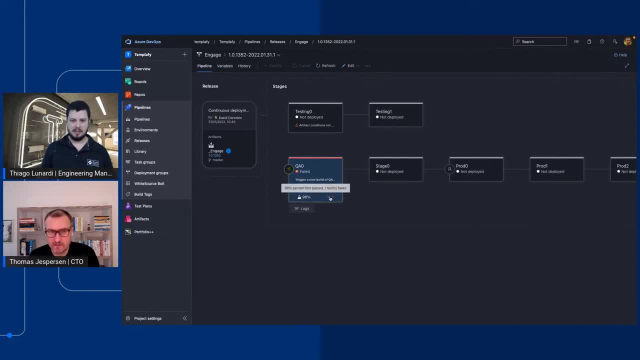 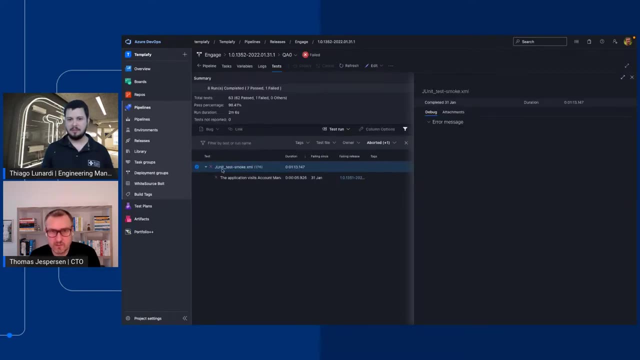 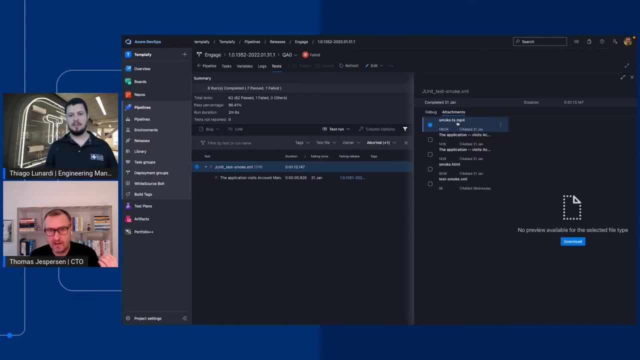 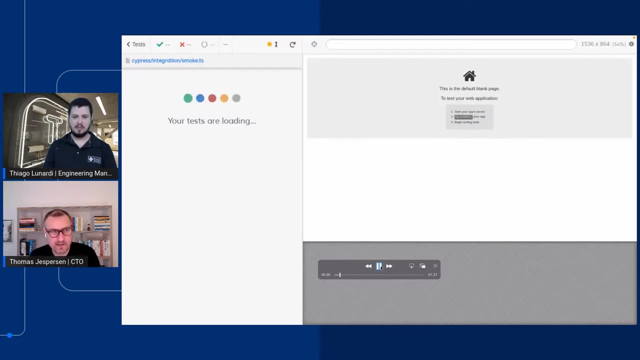 file, an MP4 file, recorded and I have actually downloaded this and I have and I'm going to play it for you. So the first thing you can see is that start by loading some tests, and then it says: okay, let me initialize a new tenant, enable all the modules, invite some users and then we'll. 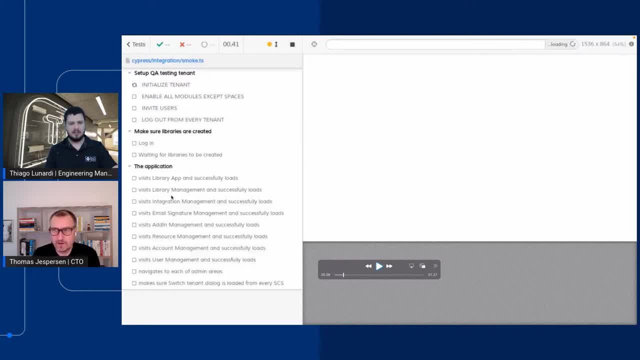 log in and we'll start navigating through the different parts of the test- Yeah, parts of the system, just to make sure once again that we didn't break anything before release it to production. And if there is any breakage, this is going to also help the engineers to debug what actually. 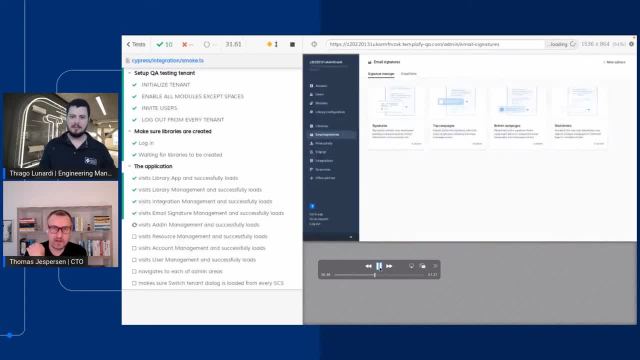 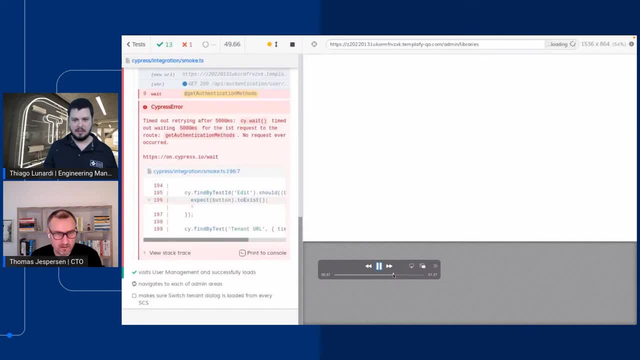 went wrong. right, Exactly. So, as you can see here, it's navigating extremely fast through our system And eventually, I think if we go in here, you will see that we have an error. He had failed. There was some timeout. 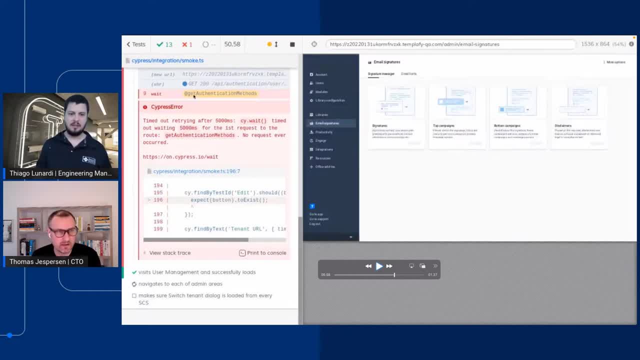 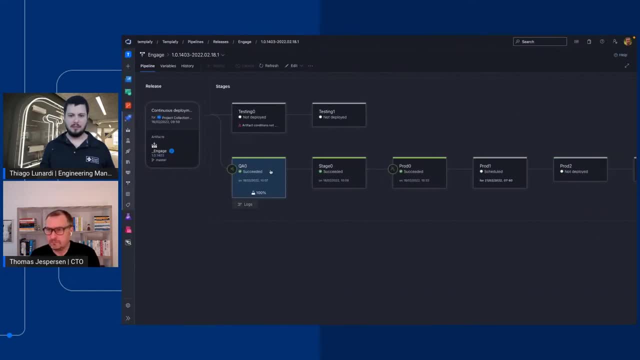 And now the engineer can say: okay, it seems like it's called get authentication method, and then they can use this to start debugging the system. So, coming back to the original release, it's now deployed to QA. We have the end-to-end testing. 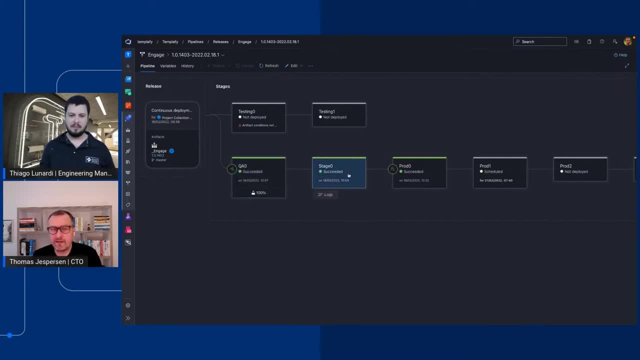 Then we deploy it to a staging environment where we can do some final regression tests. So this is the last place where engineers have a chance to actually stop the release And when they're happy, They can click on approve. So this is something that happens when they get an information or message on Slack, where 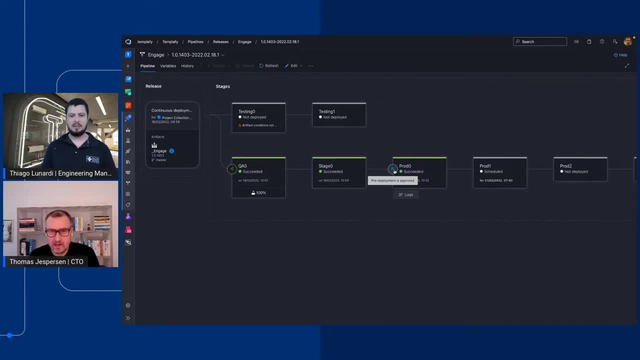 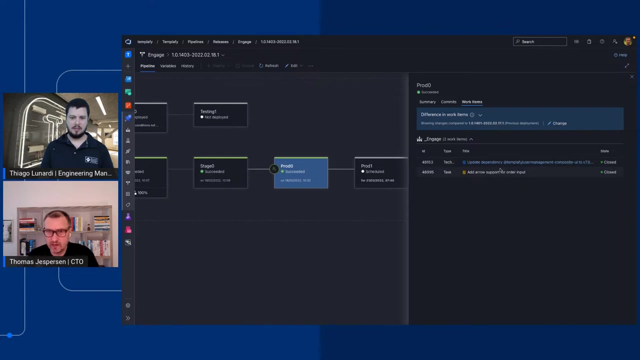 they can just approve it directly from Slack And again, when we click this approve, it will then kick off a release to production And when this happens, it will take the work item that is behind this release. And actually you can see there's two work items in this one. 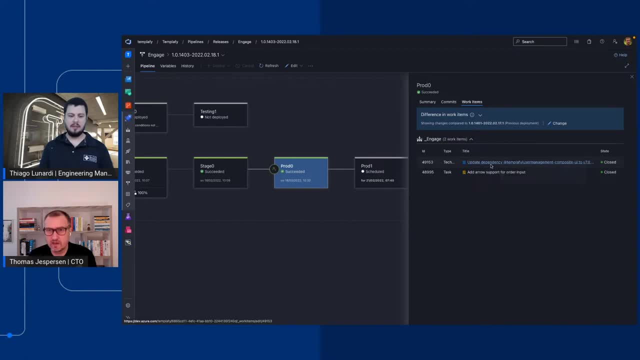 So it started out by kicking off by one, but then it ended up by two. This is the end. This is how I got confused before. So it's actually releasing two things, But these work items automatically will move to close when we get to this place. 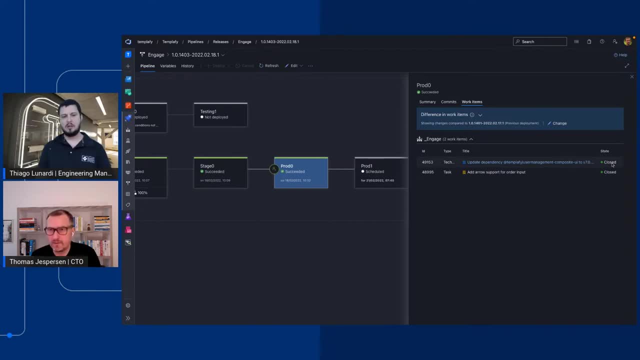 And then the release notes are published to our wiki at this point Automatically, Right, So as soon as we approve it's released Work items, Close it. Exactly, Job done. And now we said that we are doing deployment, I think, like 20, 30 times per day. 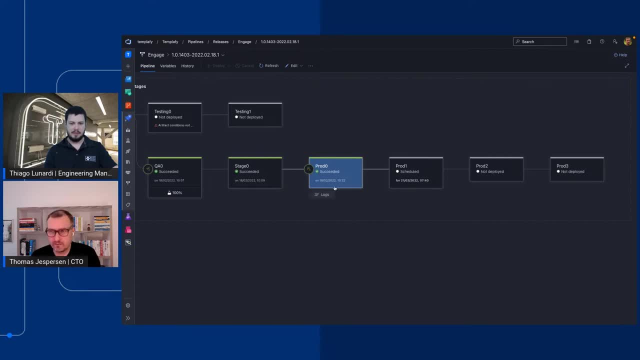 Mm-hmm, And we are actually only deploying to what we call prod zero. And this is where we run our own tenant for Templify, We run our partner tenants, We run our demo tenants, But we also run a lot of real customers, but only-. 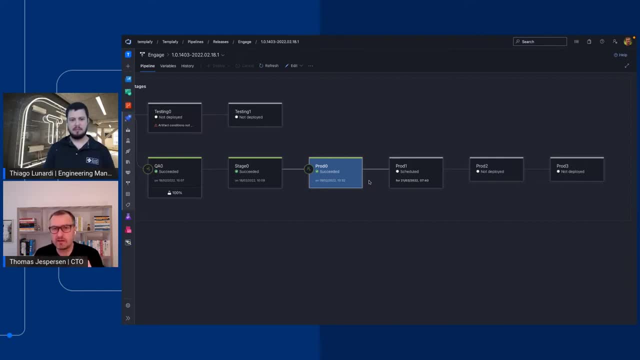 Small ones, Only the small customers. The big enterprise customers are running on the other environments here And, as you can see, this deployment was three hours ago, Mm-hmm. And tomorrow, actually, it's Friday today, so tomorrow is Saturday. 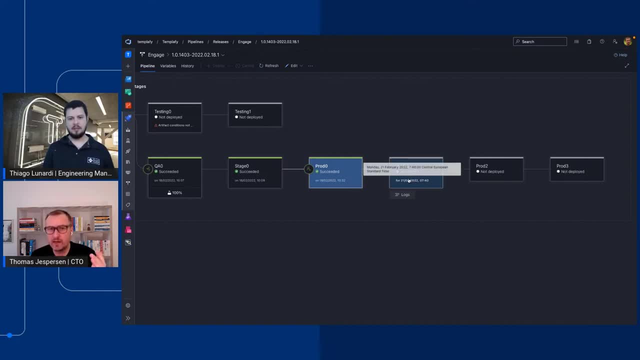 So normally it's the day after, but this is on Monday, and Monday it will be deployed to one, two and three And these clusters here- And what are those things? Yeah, Yeah, So this cluster here is running in Europe. 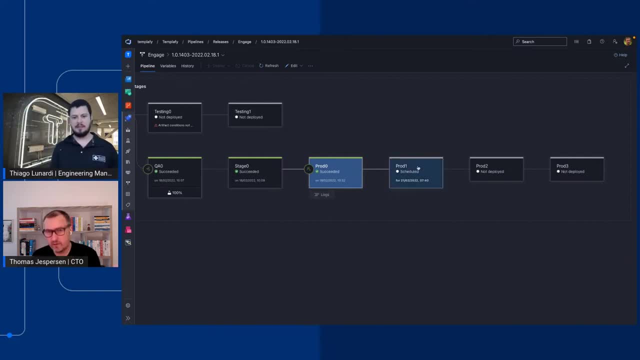 By the way, this one is also running in Europe. So both zero and one are running in Europe, two is running in US and three is running in Australia, Nice And, as you can imagine, we could add South Africa. Yeah, 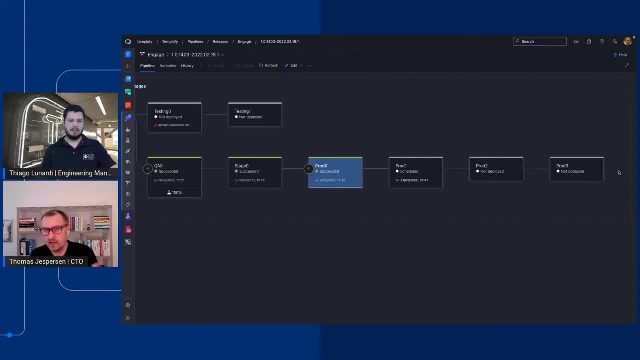 Yeah, We could add South America here, And as we grow we will probably add more and more clusters. so we can deploy, And most probably with really low effort because, as you mentioned already, we are working with Terraform, which you can just release infrastructure as a code and then just attach. 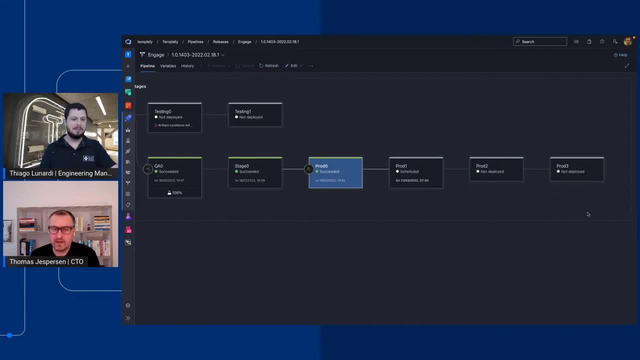 one more cluster here and it's exactly released, right, Exactly, And this is also all automated. so this is something we will probably show you in a later episode, how we built this. So spinning up a new cluster is literally just a few configuration parameters, and then 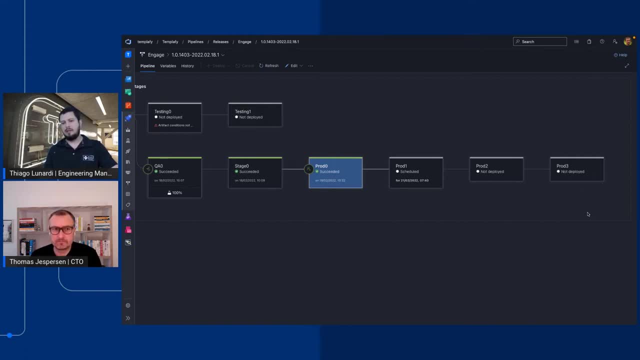 boom, Here we go. May I make one question: If we have a situation that I have a bug that was discovered in production and then released, do I need to wait until the next day to have it released to Europe, US and Australia? 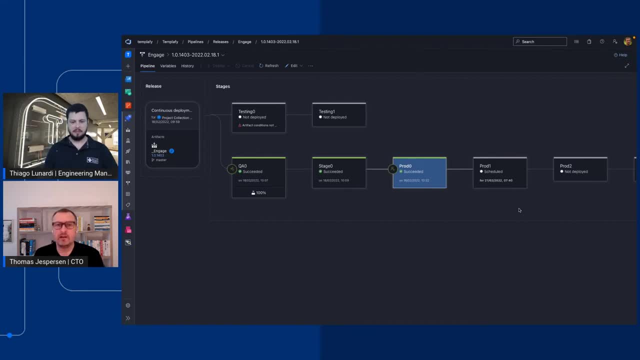 So if a bug is marked as high or critical, or if it's an incident, we will just push it directly to all the different clusters, Because this is just a safeguard. It's just a safeguard to make sure that if there is a bug or an incident, we will most 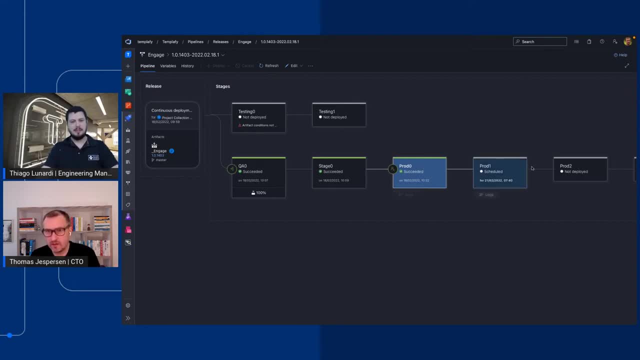 likely find it on Prot0 before we push it to the other environments. But if we find a problem here, we will fast forward all the way up, And the thing to say to us is to mention is that we don't roll back. What we do is that we do a patch forward. 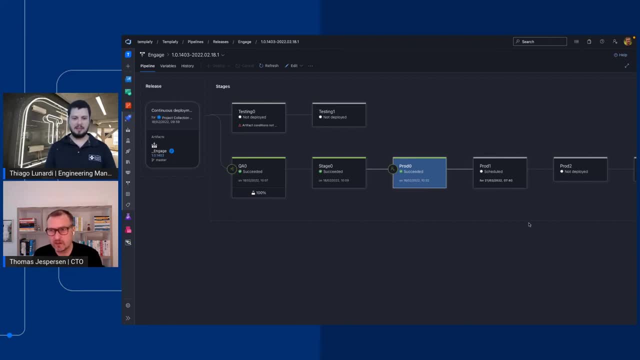 So we do this deployment many, many times per day. Everyone knows how to do it, As I just showed you. it's pretty safe. So when we have a production incident and want to fix that, we just roll forward. This ensures that if we have, for instance, database schema migration, so we make a deployment. 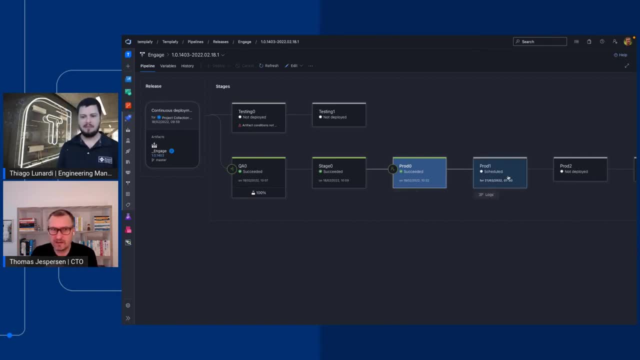 where we add a new column and so on. then when rolling back, then the column was there. So it's really complex. to roll back while rolling forward, so to speak, is something we do 20 times a day, So we know how to do that. 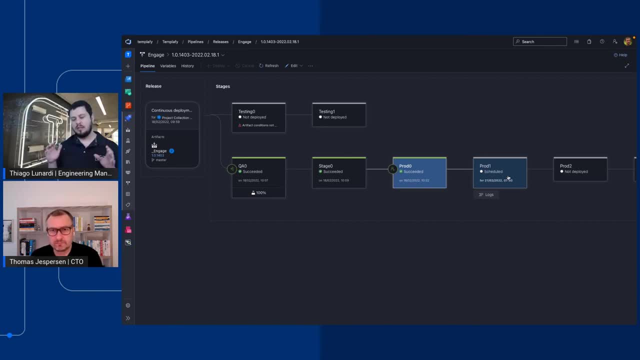 Nice And for the last, All this process here looks like a real mature and stable and on, Is there any room for improvement? All of that, Yes, definitely. I mean one of the things, as you probably already picked up, is that we run the end. 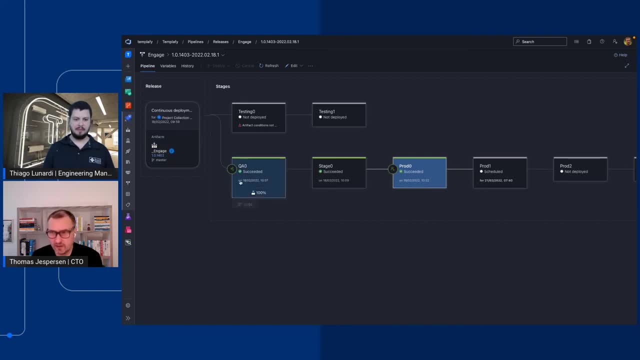 to end test both on the feature environments and on QA, And we have some regression testing here. But the plan is actually to skip these two steps here, because we already did this on the feature environment, So we have been moving to one. So what's this? 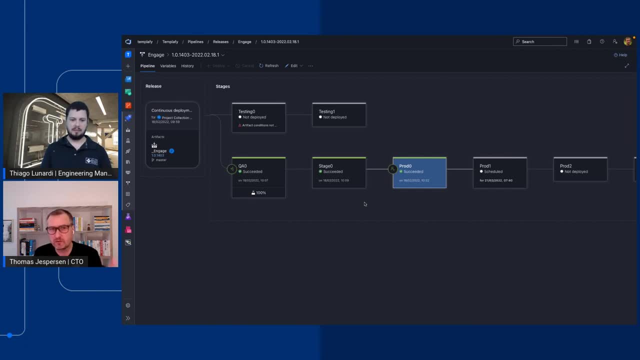 We just want to make 100% sure that it's stable and we can trust the feature environment to find all the regression box we might introduce. And then we can skip these two and also this approval, So we will push on green. So that's the difference between continuous delivery and continuous deployment, where 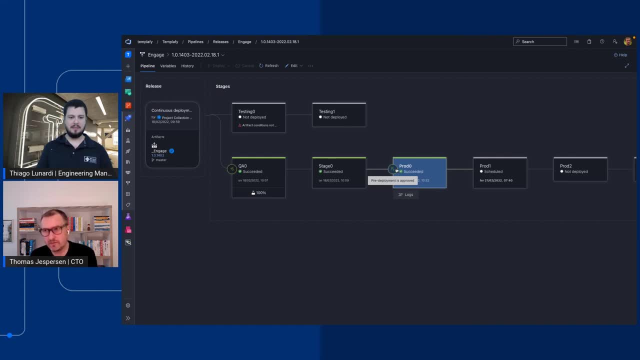 you simply just push directly to production when it's green. So this is definitely a pull request, is going to be fully approved and in green and all tested, We just ship it to production Exactly. So that's, that's one of the optimizations that we are going to do. 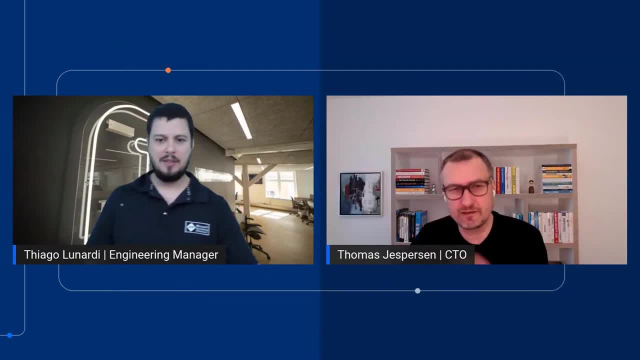 And we have been working towards that for quite some time and we are this close, Cool. Thank you very much. Everything was really really cool. Who would like to say some last words before we wrap it up? Only stick around, subscribe to the channel.